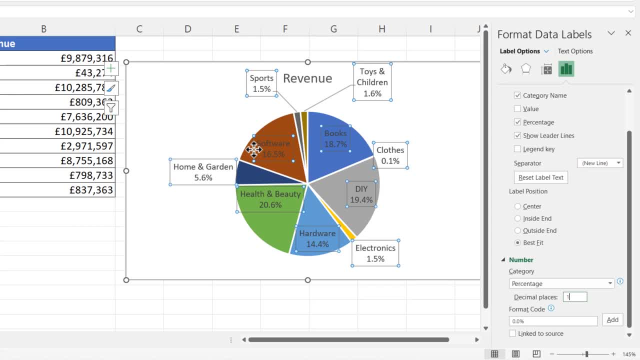 change the font color of the label. Now you need to be careful that when you do this, that you only have the particular label that you want to format selected. You can see at the moment that all of the labels are selected, but if I click on that label again, it deselects. 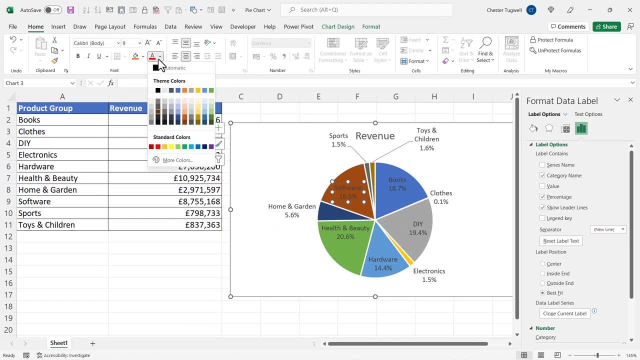 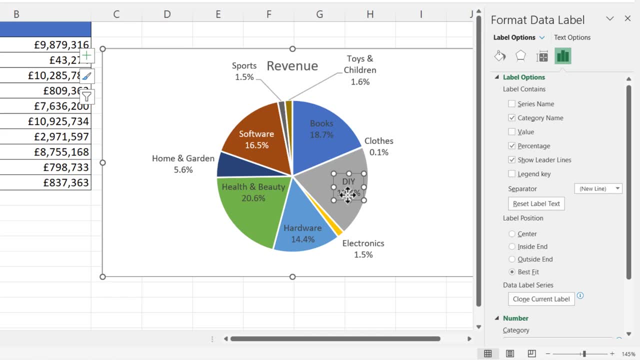 The others. I can then go to home, change the font color to white, Your other option, for example. I'll do this for DIY. If I select it and none of the other labels are selected, I can drag it out and it will then appear outside the segment within the pie chart. 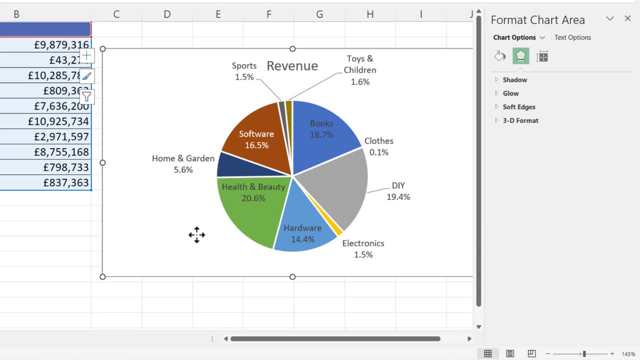 If you want to emphasize one particular data point within the pie chart, let's say software, what you need to do is click in the pie chart and then click in that segment again and then drag it out, and that will explode that particular segment within the pie. 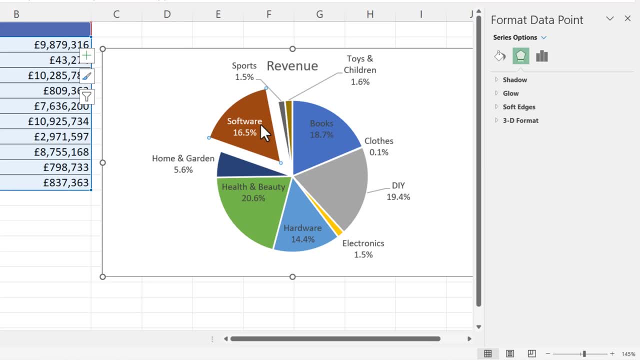 chart. now the other thing you can do is display your data in a pie of pie charts, and this is quite useful when you have data points that are quite small compared to the others. now we have that scenario. for example, clothes only represents 0.1 percent of the data. you can't actually see it. 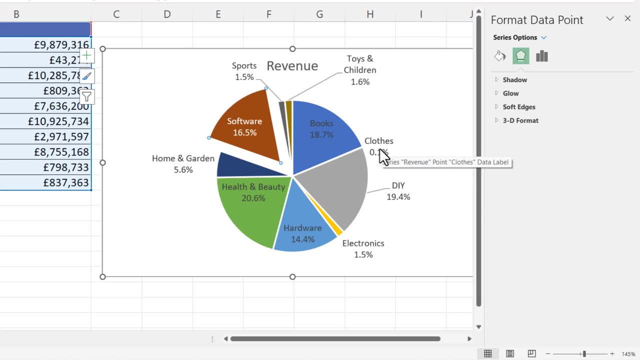 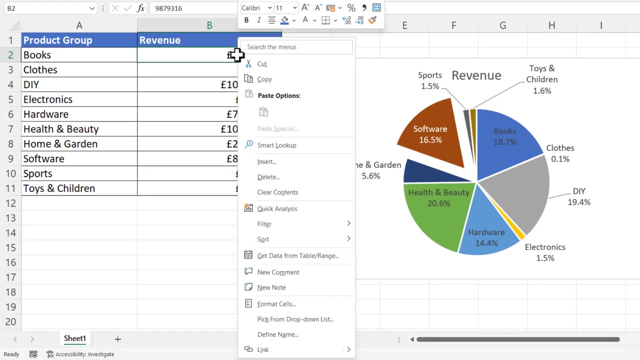 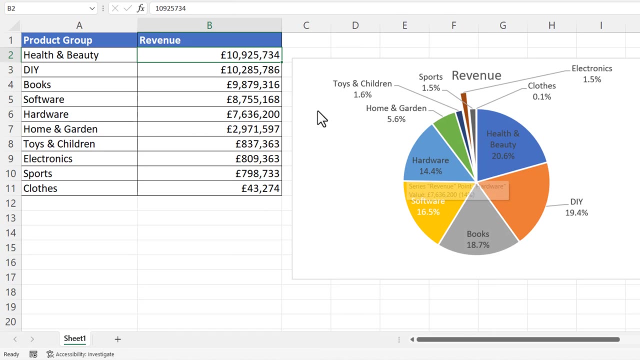 in the pie chart at all, even though you have a label there. so what you should do is first of all get these values in descending order, the revenue values in this example. so i'll right click in one of the revenues. i go to sort largest to smallest. then what you want to do is change the type of 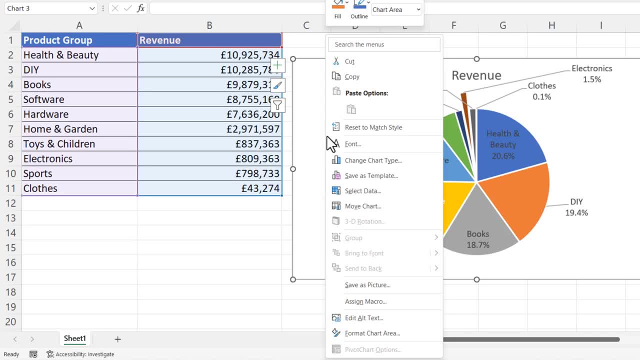 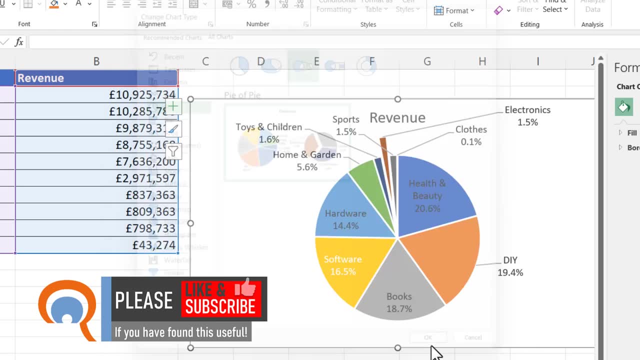 chart that you're creating. so if you right click in an empty space in the chart, you can go to change chart type and select this type of chart: pie of pie. click on ok and what it will do is it'll put the smallest values in a secondary pie chart and it'll put them in a secondary pie chart. 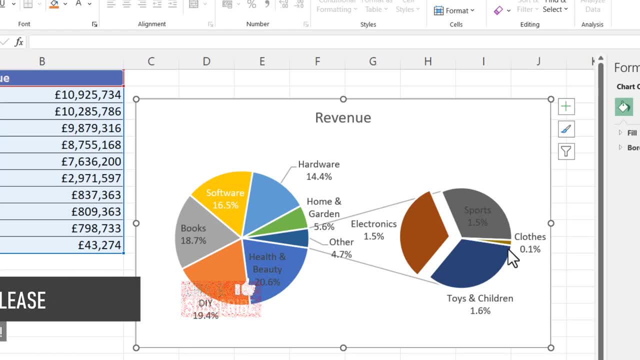 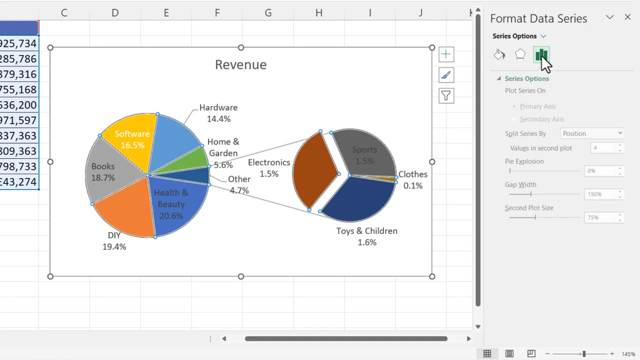 chart. so we can now see the clothes data point and you can see that all of these data points in this secondary pie chart are represented by the other segment within the main pie chart. now if I click into the main pie chart and I then click on this button over here- series options- I can change the number of values that 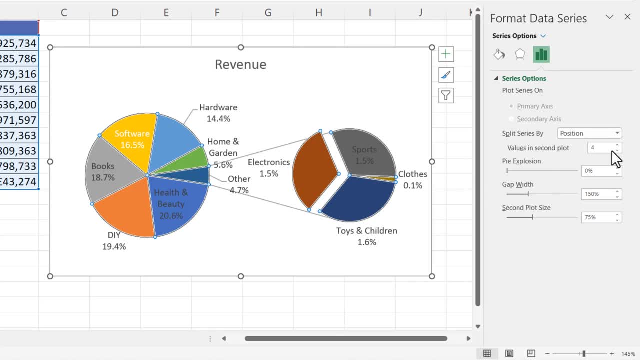 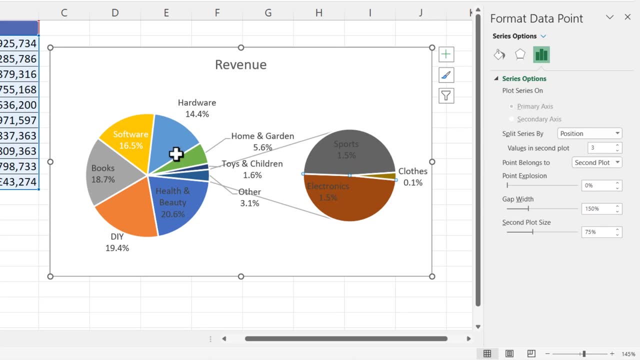 appear in the second plot. at the moment, we have four values. if I increased it to five, you see that that's still exploding. let's drag that back in, or I could decrease it to three. so you have a lot of control in terms of which data points.